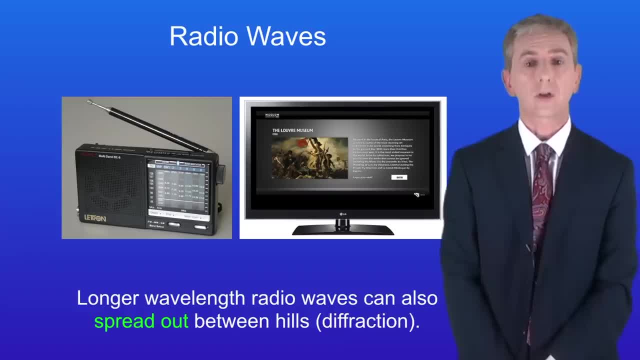 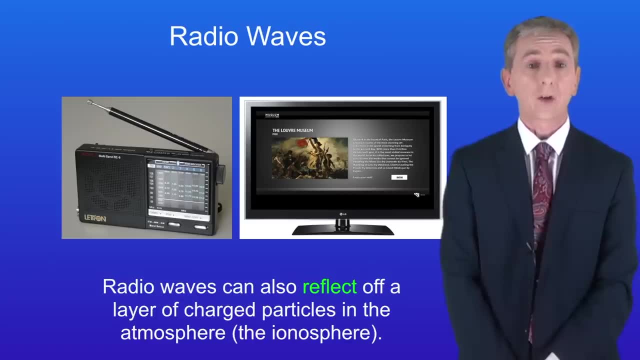 waves can also spread out between hills, and that's called diffraction. I should point out that the word diffraction is not on your specification. Radio waves can also reflect off a layer of charged particles in the atmosphere, and that's called the ionosphere. This allows us to send. 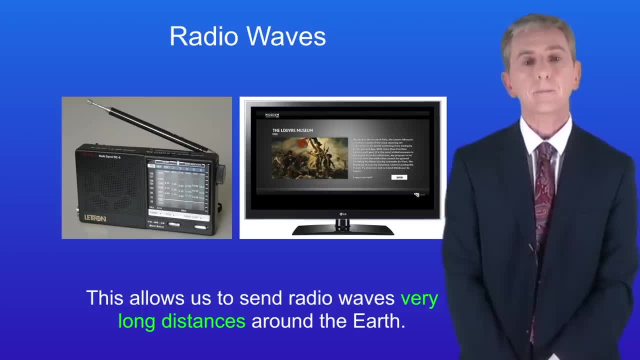 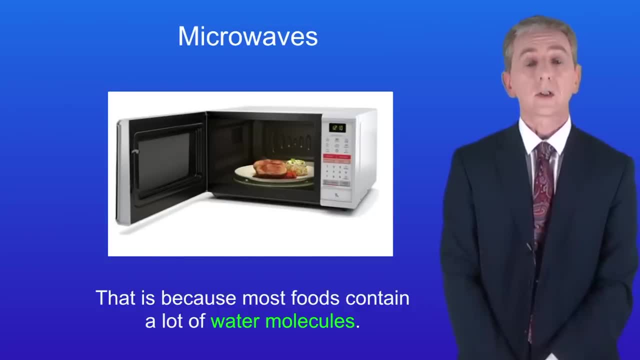 radio waves very long distances around the earth. Okay, let's look at microwaves. Firstly, microwaves are used for heating food. That's because most foods contain a lot of water molecules and water molecules absorb the energy of microwaves. The energy causes the temperature of the food to 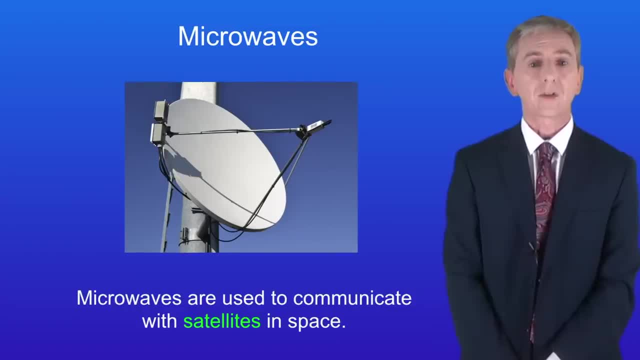 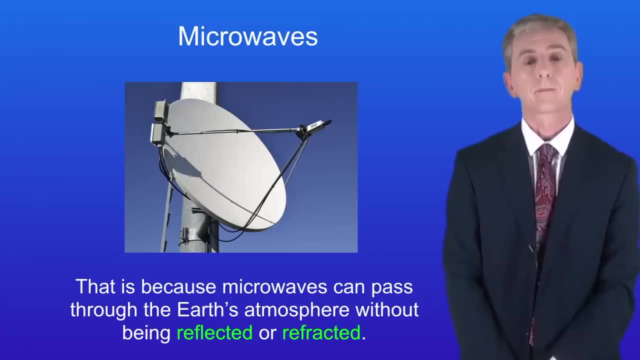 increase. Secondly, microwaves are used to communicate with satellites in space, and that's because microwaves can pass through the Earth's atmosphere without being reflected or refracted. Okay, we're going to look now at infrared. Infrared is emitted by electrical 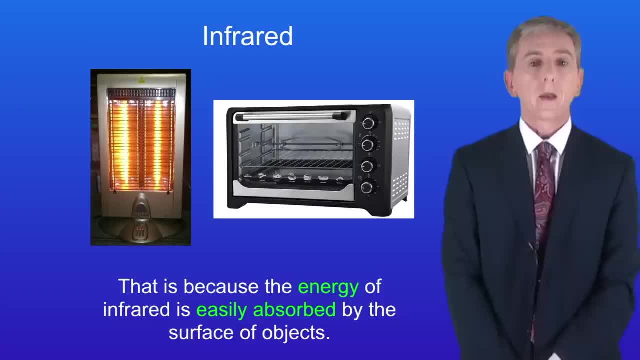 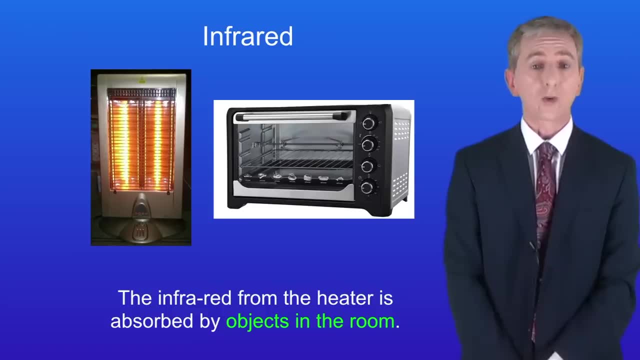 heaters and it's also used to cook food in ovens. That's because microwaves are used to heat food? That's because the energy of infrared is easily absorbed by the surface of objects. For example, the infrared from a heater is absorbed by objects in the room and this makes the room warmer. 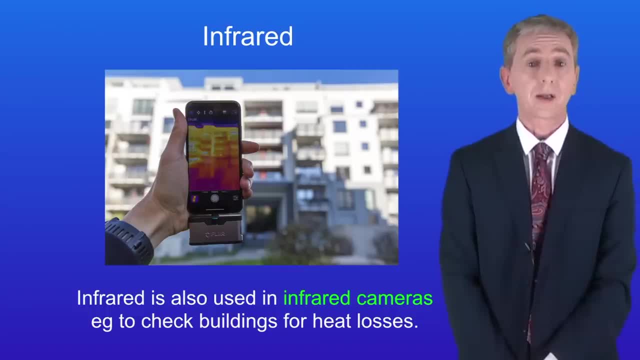 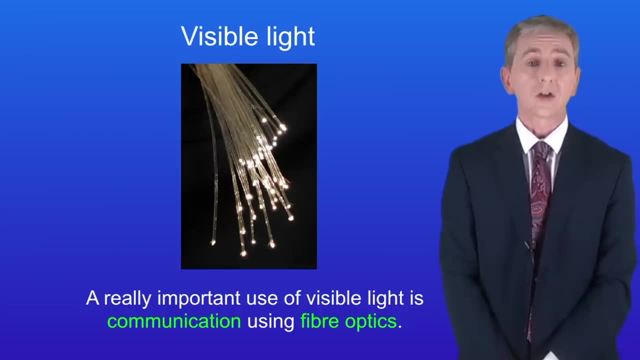 Infrared is also used in infrared cameras, for example to check buildings for heat losses. Let's look now at visible light. A really important use of visible light is communication using fibre optics. I'm showing you here a bunch of optical fibres. Optical fibres are very thin strands of glass We can transmit. 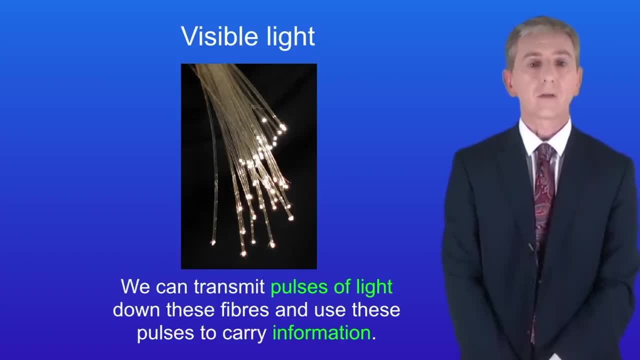 of light down these fibers and use these pulses to carry information. Optical fibers are used to carry telephone and cable TV signals. Now, because visible light has a short wavelength, it can carry a great deal of information. Okay, the next electromagnetic wave is ultraviolet. Now a. 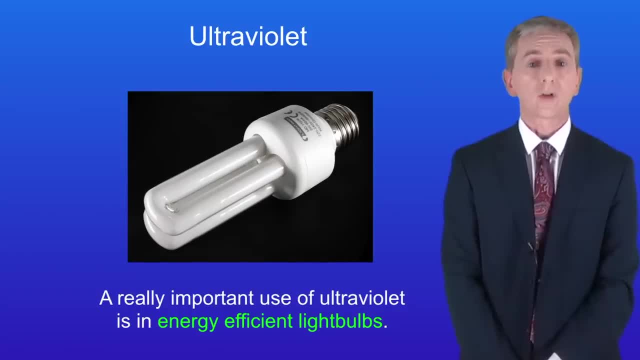 really important use of ultraviolet is an energy efficient light bulb such as this one. Ultraviolet light is created inside the bulb. Now, because ultraviolet has a short wavelength, it carries more energy than visible light. The energy of the ultraviolet is absorbed by the internal surface. 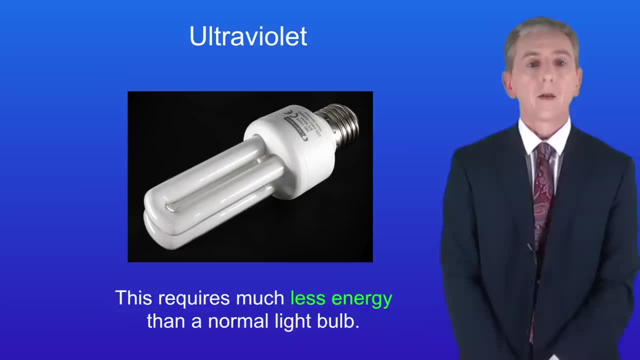 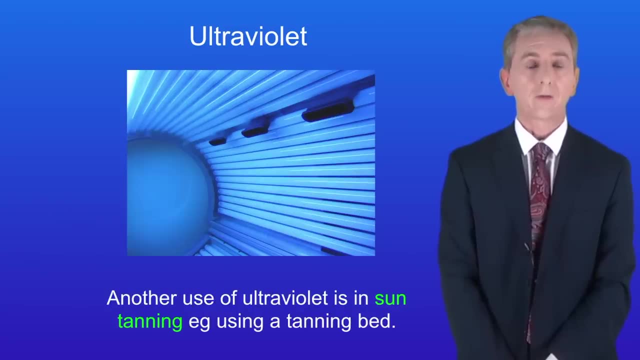 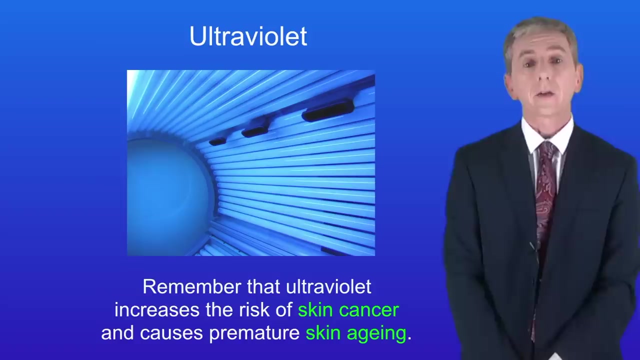 of the bulb and it's converted to visible light. This requires much less energy than a normal light bulb. Another use of ultraviolet is in sun tanning, for example, using a tanning bed such as this one. However, remember that ultraviolet increases the risk of skin cancer and it causes premature skin.